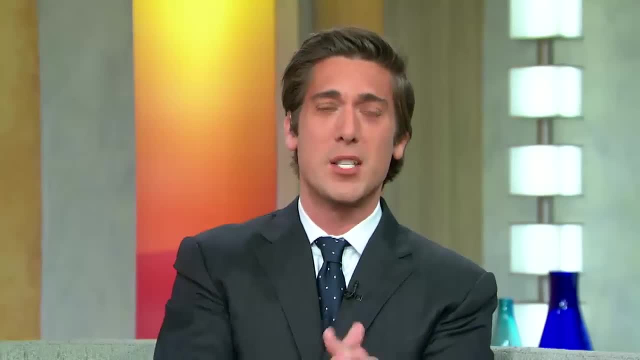 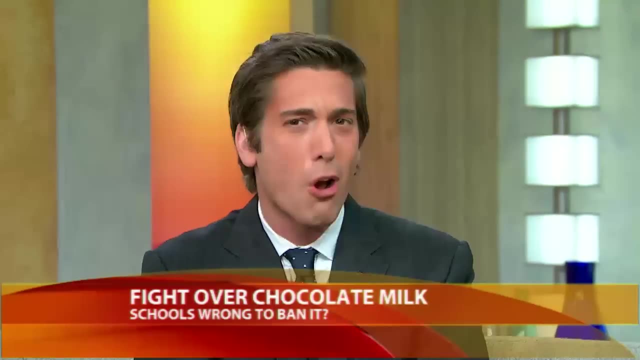 Big debate. Parents and kids are going to put down the backpacks this morning. They're going to want to weigh in on this, because the question is: schools across this country are really trying to make their lunches healthier, safer for kids. The question, though: should chocolate milk be saved? 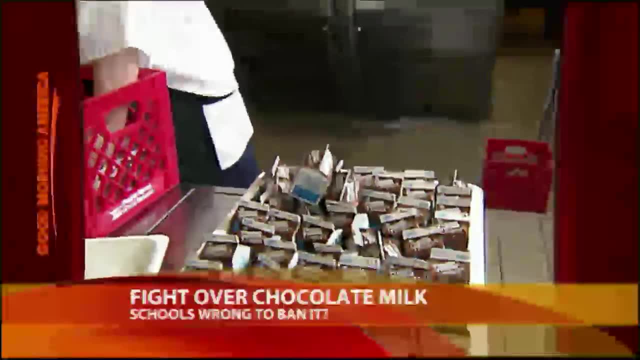 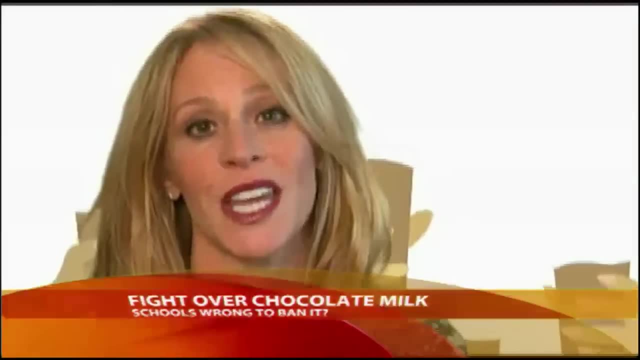 It's been a staple of school lunches for decades: chocolate milk. And the dairy industry is now fighting to keep it that way, as many schools look to make their menus healthier. Unfortunately, a lot of schools have taken chocolate milk off the menu. 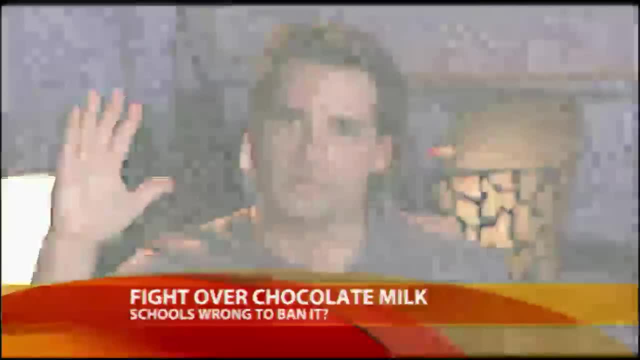 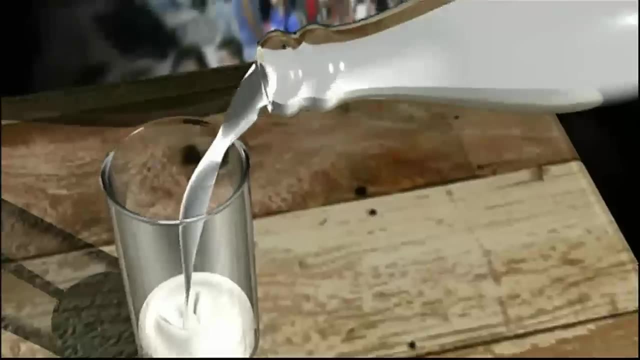 This morning the dairy industry is launching a campaign spending, by some estimates, nearly a million dollars to make its case. I like chocolate milk and I know my girls will too. On one side of the debate, chocolate milk is too fatty: 12 grams of sugar in a half pint of regular milk. 24 to 30 grams of sugar in chocolate milk. 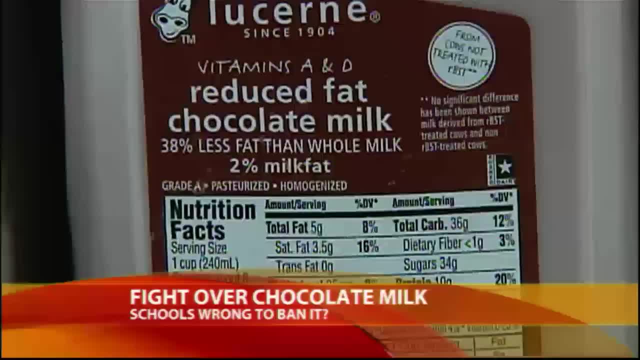 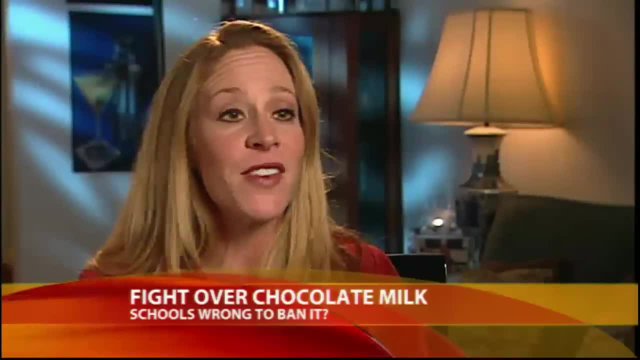 But defenders say that extra sugar is worth it, given the calcium and the vitamin D benefits children need. When chocolate milk is made available, kids will pick it, they will choose it and the benefit is that they're getting the nine essential nutrients. 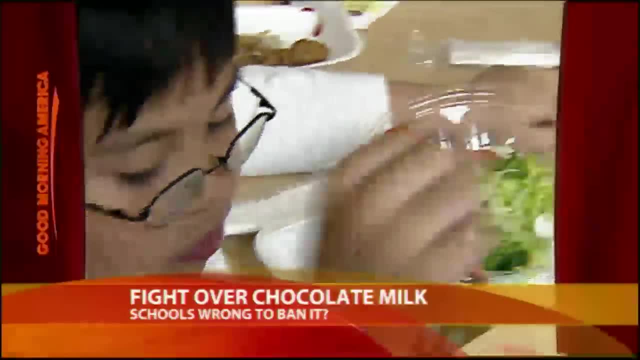 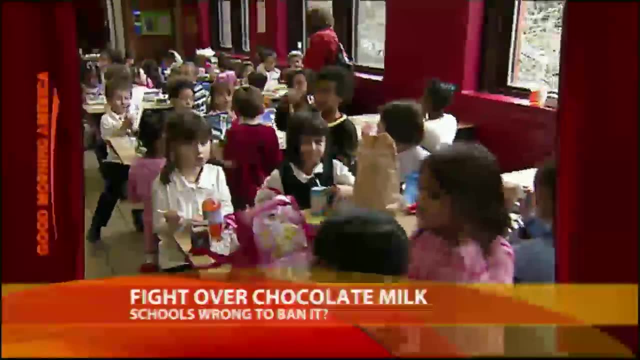 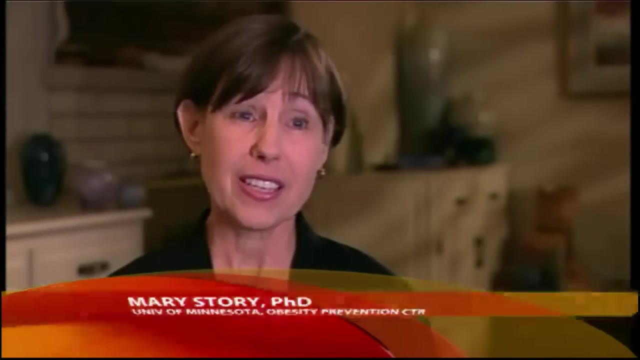 But some nutritionists say schools dropping chocolate milk are simply being smart about all that sugar. When children have chocolate milk on a daily basis at school, it's really going to be hard for them to go back home or just to be drinking plain milk. 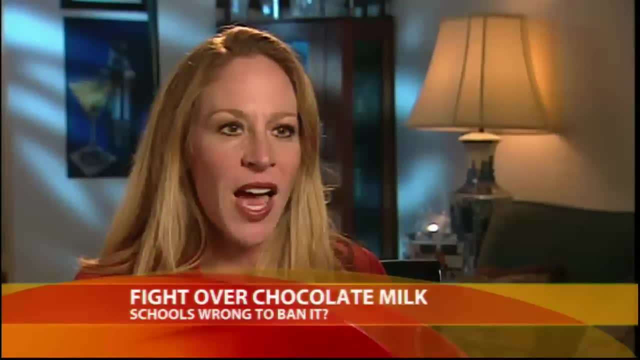 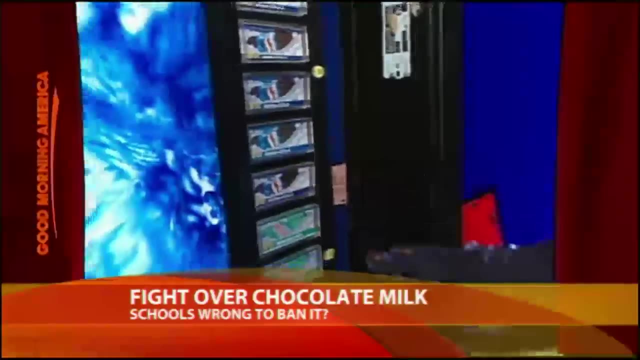 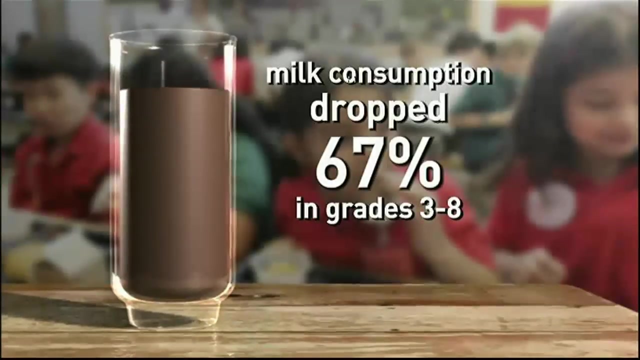 If you take chocolate milk off the menu in school cafeterias, then what kids are left with are other sugary beverages that have no other nutritional value other than calories. In fact, A recent study of a Connecticut school district showed when chocolate milk was taken away, milk consumption of any kind dropped 67 percent in grades three through eight. 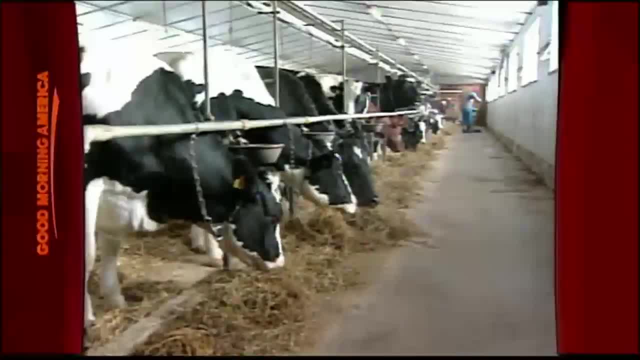 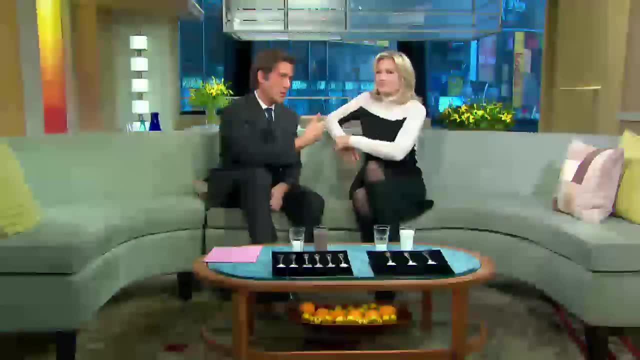 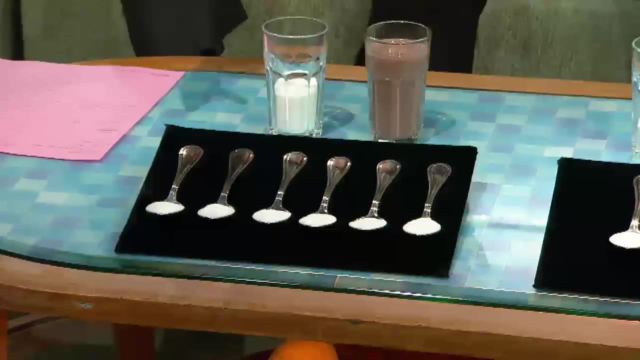 Chocolate milk defenders say: look at all that nutrition lost, while critics say the dairy industry is looking at all the money lost. So we were saying during the piece: how much sugar are we really talking about? Take a look at this. This is a typical chocolate milk at lunch and you're getting about. well, they say three teaspoons with white milk, six teaspoons of sugar. 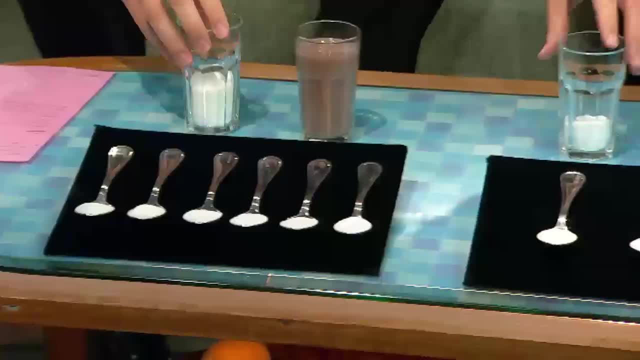 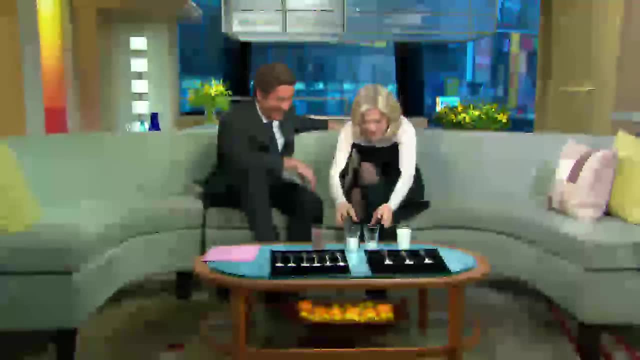 And this is actually the sugar piled up in the glass. So put this next to the sugar that you get in the regular milk and that's the difference. The question is, I'm trying to measure them here, But what are the alternatives at school? 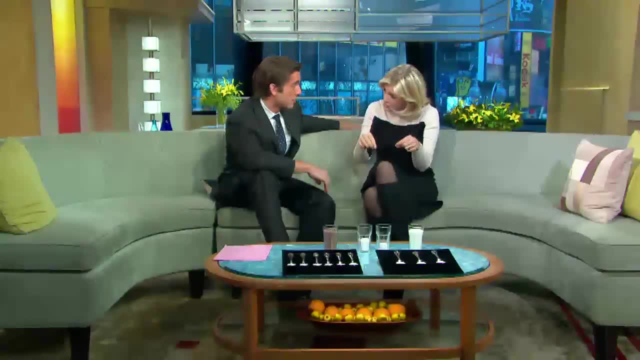 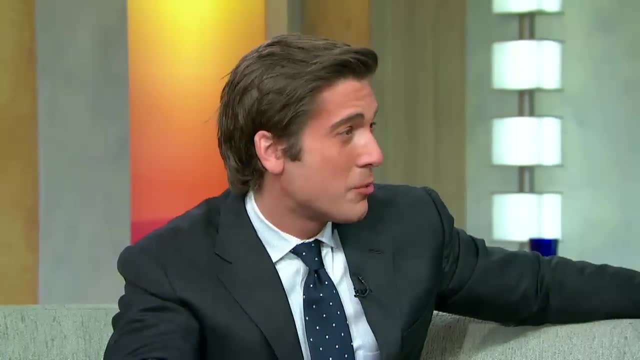 I mean, if they're not going to drink the regular milk, they'll drink juice which also has some sugars in it- right, It has sugar- or drink nothing at all. And so parents would say: if I want them to get the vitamin D, the calcium, the potassium, then let them drink the milk.